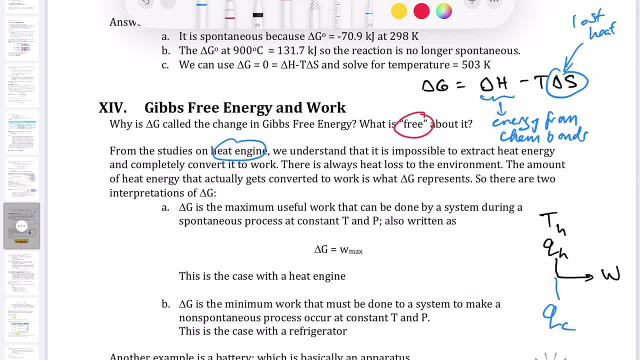 that happen, that there's a certain amount of heat that's lost And we call that QC, And there's some quantity of it that goes to work. So it might, you know, 70%, 30%, it might be 60%, 40%, It depends. 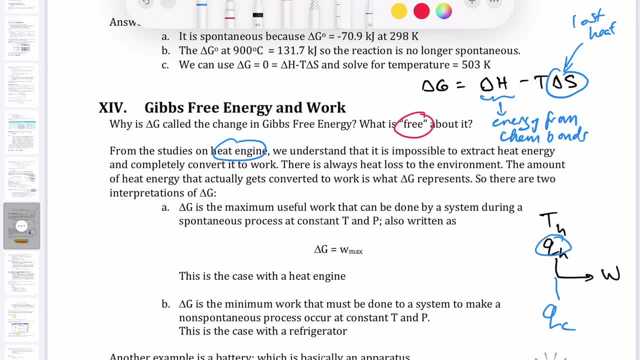 on the specific engine, but never is it possible to take 100% of the heat being generated and convert that to work, And so that's what entropy originally is. It's a quantity that captures the QC. So this work, then, is what delta G is capturing. So delta G is a quantity that captures the QC. 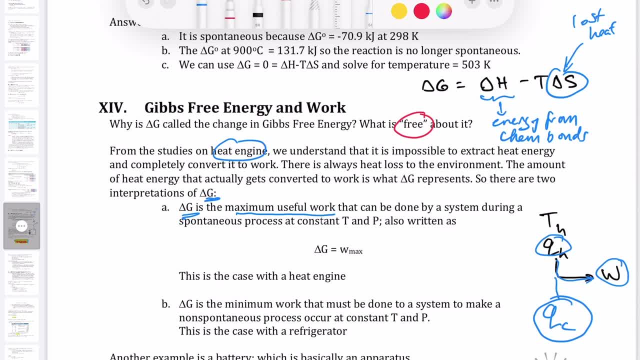 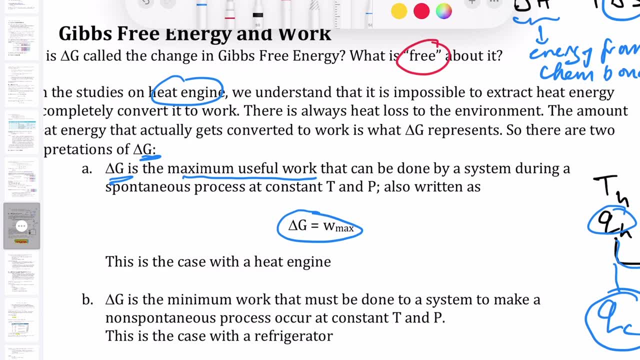 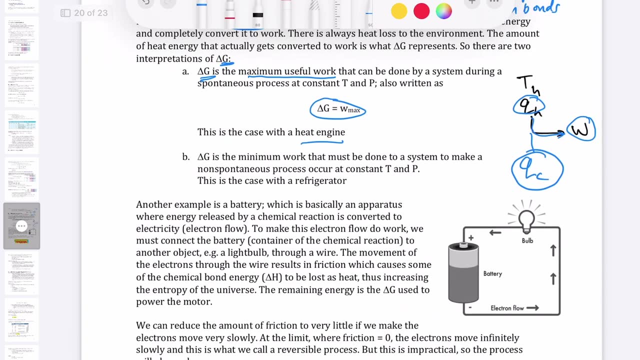 Delta G is just the maximum useful work that you can get out of a particular engine or a particular setup of a chemical reaction, And so we call delta G Wmax or maximum work. It's the case with heat engine, but it's also the case with electrical system, as you'll see in a future chapter on 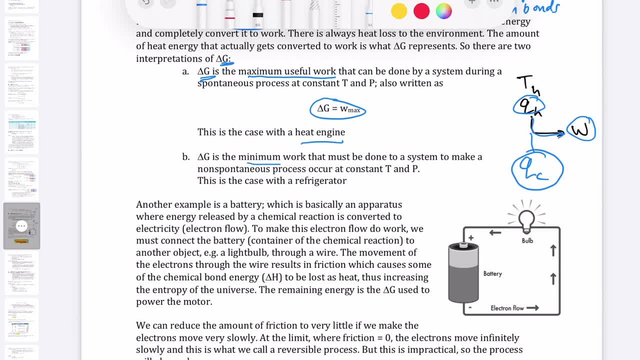 electrochemistry. Now the other interpretation of delta G is for non-spontaneous processes. It is the minimum work you have to do to make that process happen. So again, if you get a delta G, it is positive. It's basically telling you that at least you have to do that much work to get that. 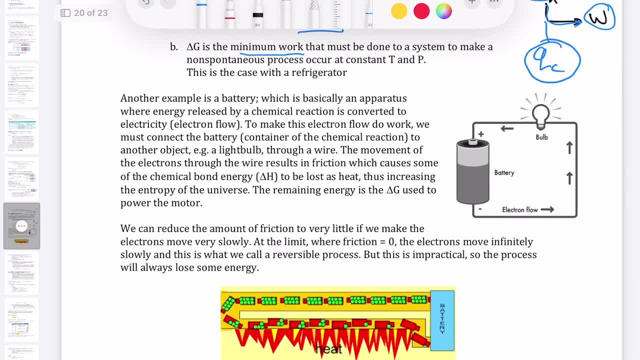 chemical reaction or that particular process to happen. Let me give you an actual example of how to visualize delta. So this picture right here shows a battery that is being used to turn on a light bulb, right So we just connect it in an electrical circuit and we can see that when it's. 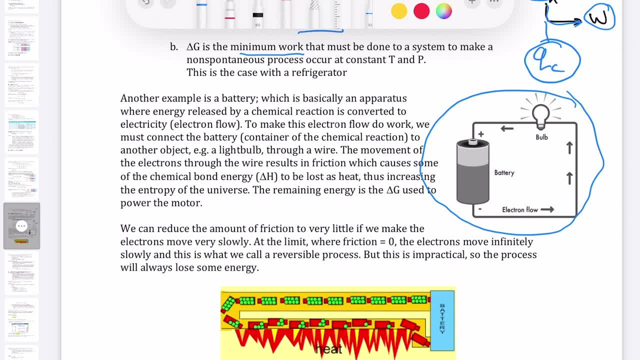 connected correctly, the light bulb will turn on. Now, how does this work? Well, there's electrons in the battery and it's moving towards the positive end of the battery. So the electron is just moving, based on electrostatic law. Now, as it's moving, anything that's moving has kinetic. 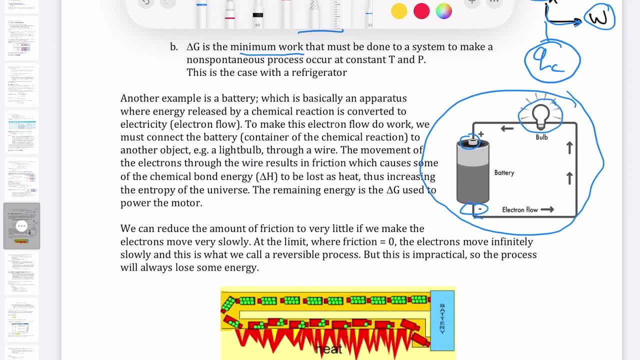 energy, so that energy could be converted into work. And the work that's done here is the work to light up that bulb, And so we see light, which is another form of energy, right, But what's interesting here is that just the movement of the electron. you would think that that could. 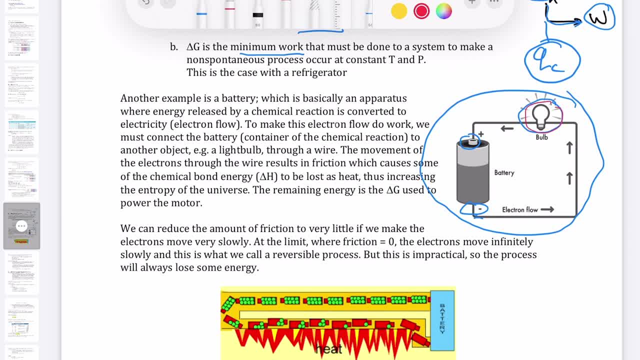 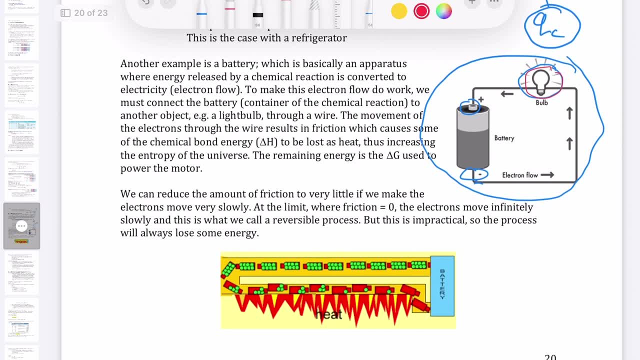 capture all the kinetic energy that the electron provides from the battery, but turns out that the light bulb actually doesn't really get all the energy from the electron. The reason is because just by moving the electron generates some friction in that material. So this is a picture of how that friction is lost through the wire. So for example, if you imagine: 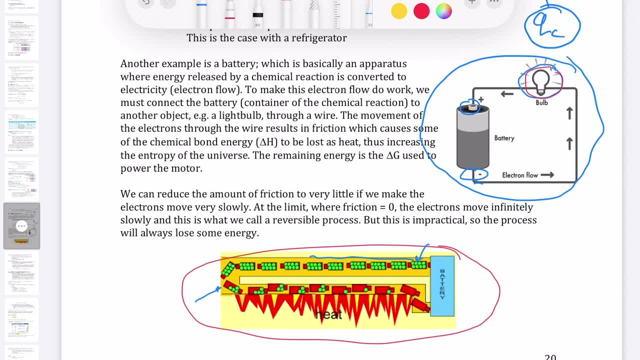 these green little dots as electrons and they're just moving around the wire. the wire is brownish cream looking color, So the electron is moving here. but as the electron is moving, they're colliding with each other And so, as a result, friction is. 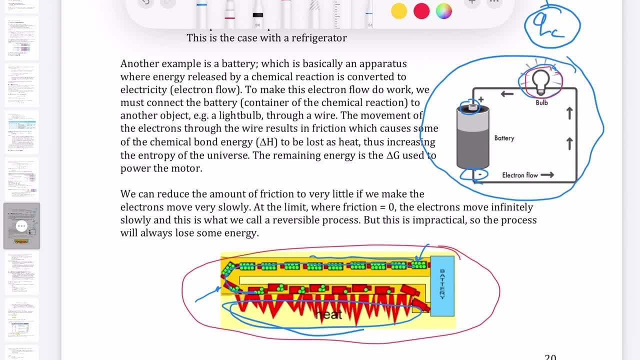 generated And so that friction is lost to heat across the wire. So if you touch a wire it has a lot of electricity, a lot of electron moving. you can feel that it's warm And that's because that heat is lost And that heat that's lost is no longer able to be used to light. 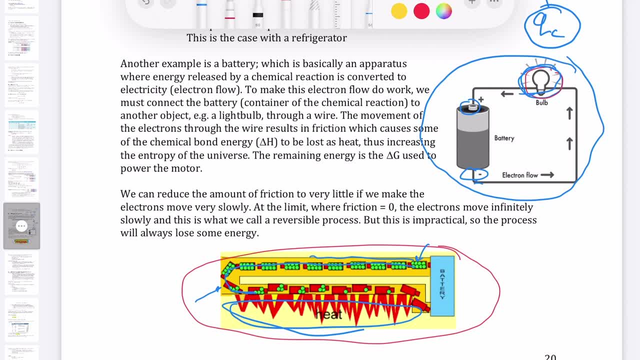 that light bulb right To generate that work. So, therefore, there's always a quantity of energy that is gone, regardless of whatever system you set up, And that quantity that's lost is your change in entropy. That's what makes the process possible to do. 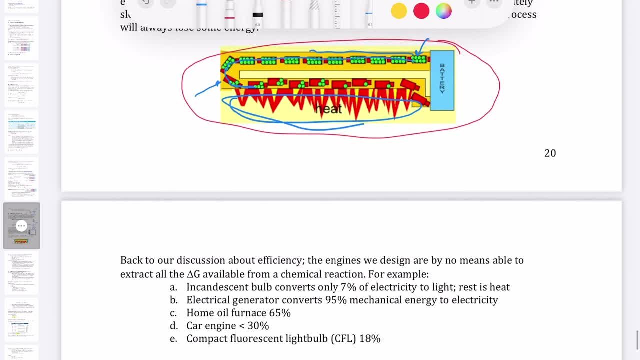 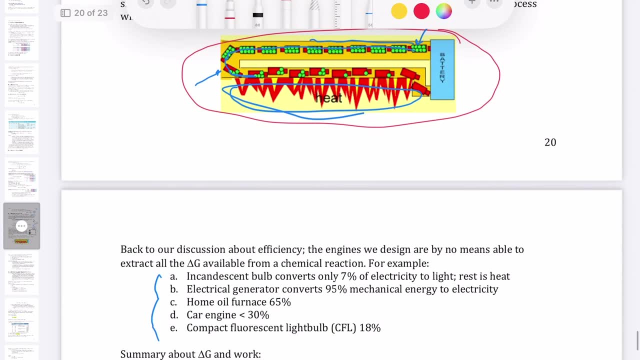 Any process you do in our universe always has this cost of entropy, And so, if we look at a lot of the different types of engines or appliances that humans have created, actually what's interesting is that we're not even able to design things that are able to capture a hundred percent. 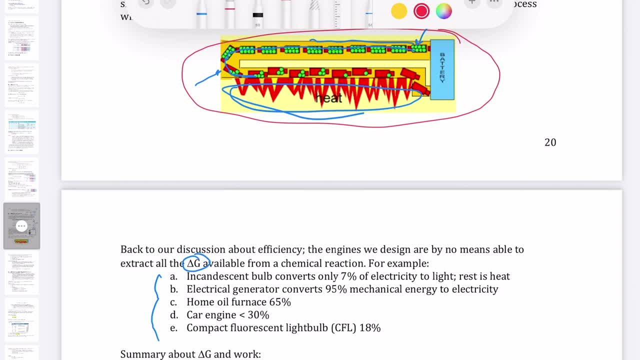 of that. Delta G Again, remember that the Delta G itself is already less than a hundred percent of the available energy right Which is given by Delta H. that energy in the chemical bond Delta G is sort of like a universal requirement that you can't get. 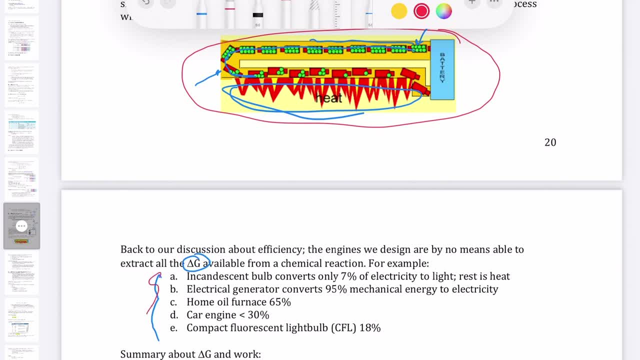 A hundred percent of the energy. But the engines themselves get even less because the engineering of these engines, the design of this engine, is such that they're not able to capture a hundred percent of that Delta G, that useful work. So here's just some examples, some numbers here to 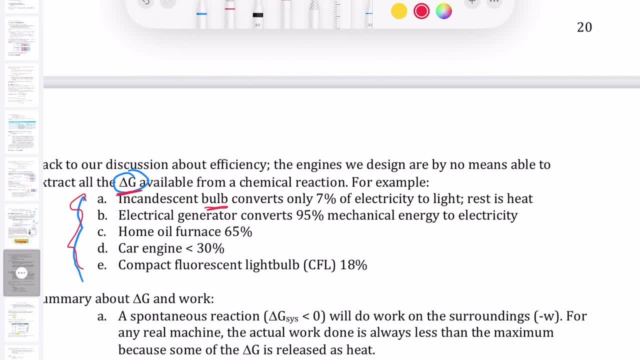 give you a little bit of an idea. like that incandescent bulb that we use for a long time- Now it's finally been taken off market- That's only able to convert seven percent of the energy from the electron flow. That's seven percent of what is possible, Okay, So it's a lot.